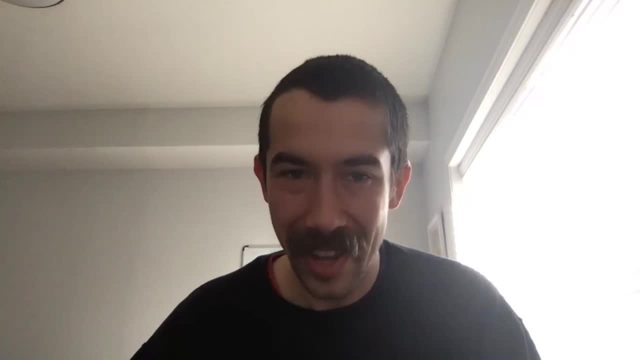 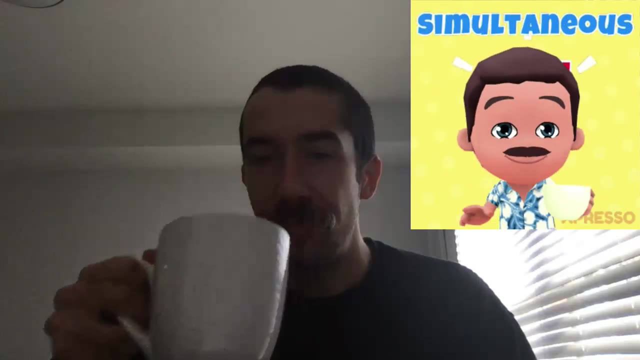 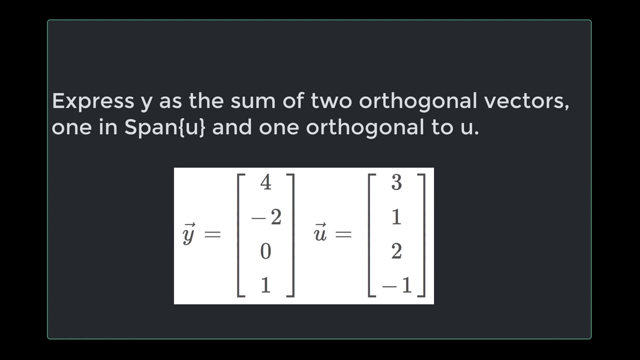 If you're ready to do math today and you have your coffee ready, join me in a simultaneous sip. The question we're working on today is express y as the sum of two orthogonal vectors, one in the span of u and one orthogonal to u, where y is the vector and u is the. 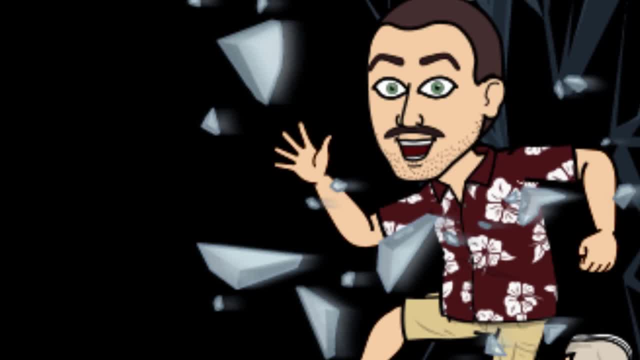 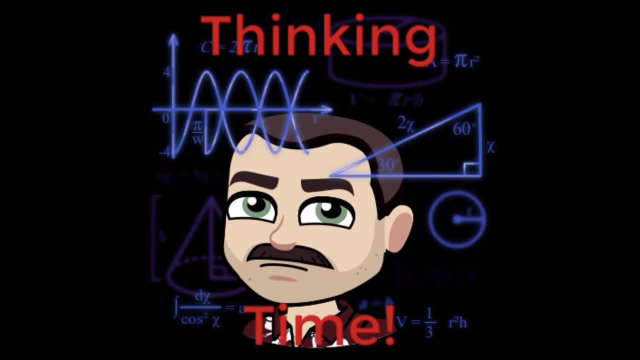 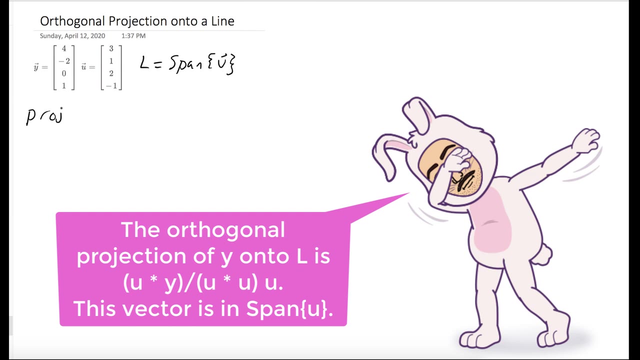 vector. Smash that like button and let's get started. So we'll let L be the span of the vector u and what we want to do is project y onto L, And the way we do that is we take the dot product u dot y over, u dot u times the vector. 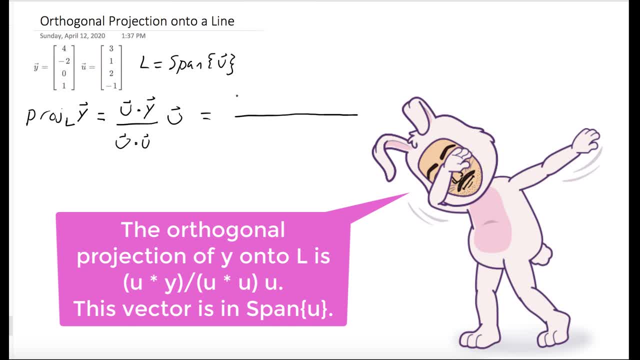 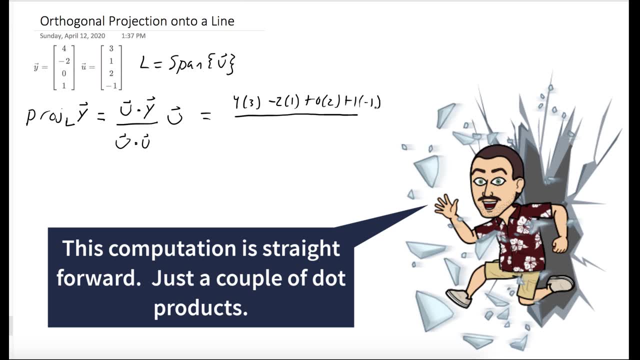 u And when we work this out? well, let's first take the dot product of u and y. We get 4 times 3, minus 2 times 1, plus 0 times 2, plus 1 times negative 1.. 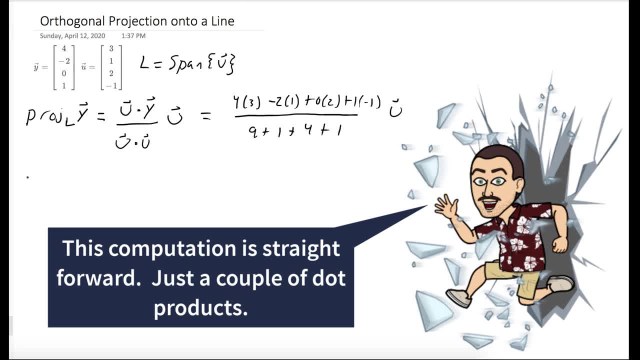 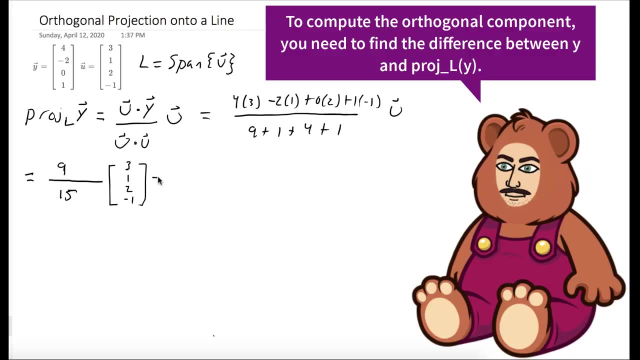 And then we'll take the dot product of u with itself and multiply it to the vector u. When we work this out, we get 9 15ths times u. And when we work this out, we get 9 15ths, 3 15ths, 6 15ths, negative 3 15ths. 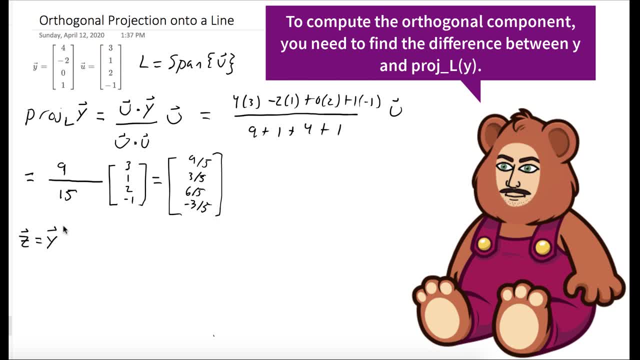 So this is the component of y that is parallel to u. To get the part that is orthogonal to u, we'll call it z and it's just y minus the projection onto L of y. So it's our vector y minus this vector that we just found. 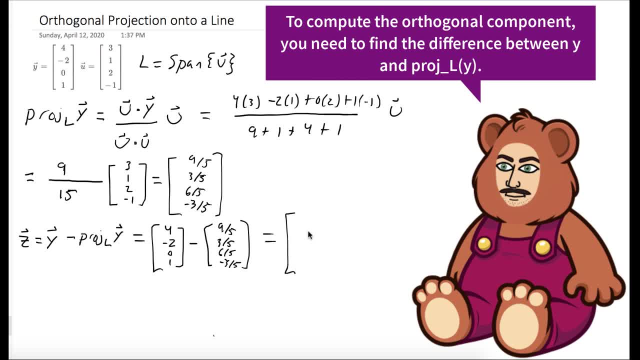 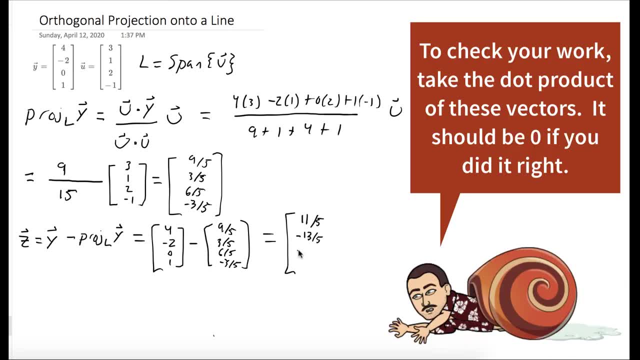 And when we work that out we get 11 15ths minus 13 15ths, minus 6 15ths and 8 15ths. So to put it all together, our vector y is equal to the first vector we found, which 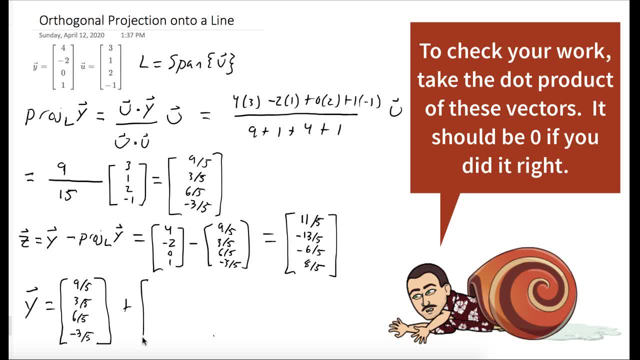 is the parallel component to u Plus the second vector we found, which is the component that is orthogonal to u.